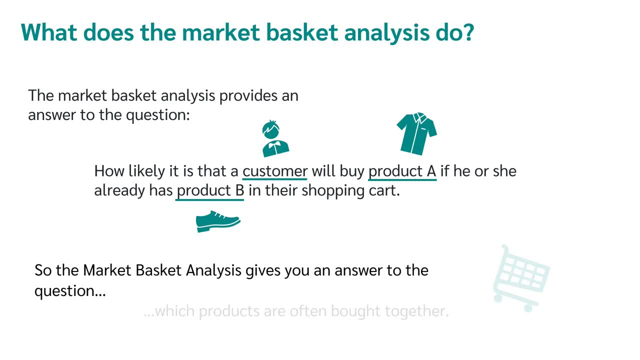 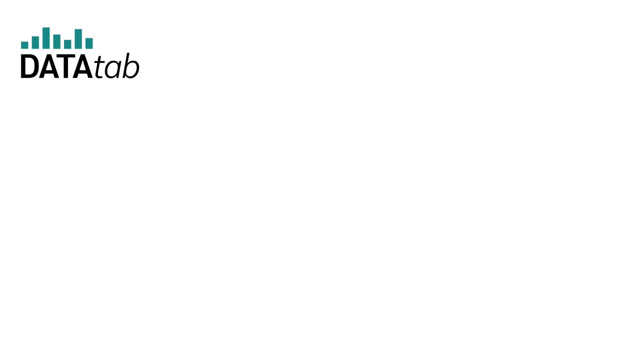 Therefore, the market basket analysis gives you an answer to the question, which products or goods are often bought together. Thus, if a customer already has pants and shoes in the shopping cart, how likely is it that this customer will also buy a shirt or socks or a t-shirt? 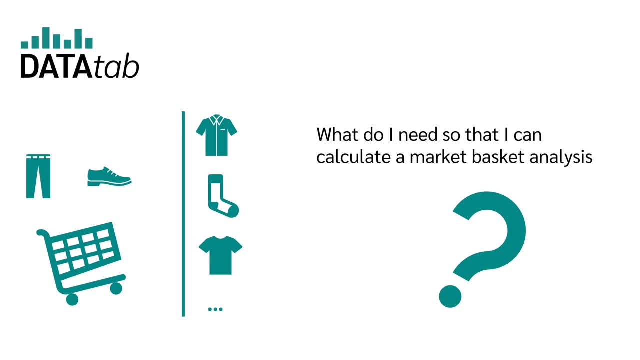 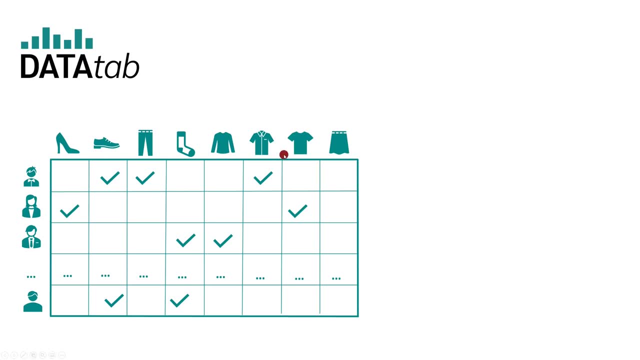 But now the question is: what do I need to calculate a market basket analysis? You need a list of past purchases in which you can see which products were bought together, So you have the products listed and each row is one transaction or purchase. 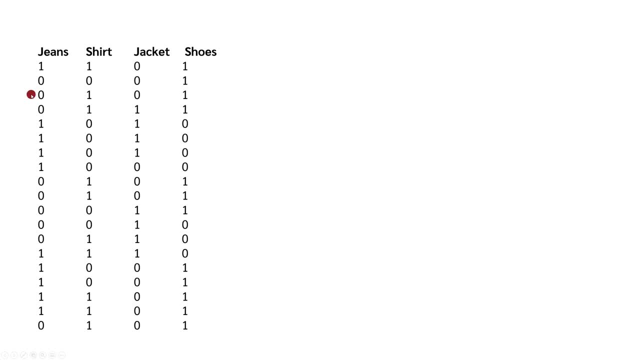 To make this clearer, let's look at an example. Let's say that this is your example data. You have the products jeans, shirt, jacket and socks. You have the products jeans, shirt, jacket and socks and shoes. Each row is one transaction or a purchase. One means bought the product Zero. 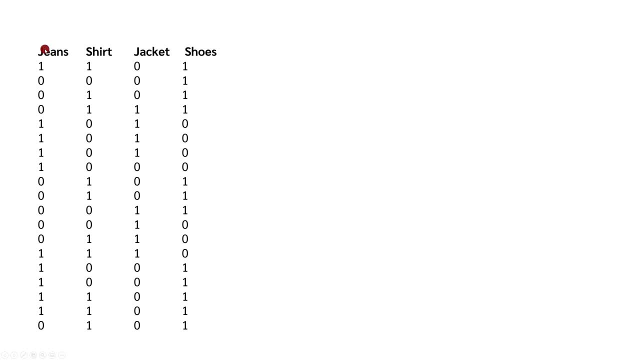 means didn't buy the product, So the first person bought jeans, shirt and shoes. If you use data depth for the calculation, your data can also be in this form, So each row is a transaction and the purchased products are simply separated by a comma In order to get results that we can. 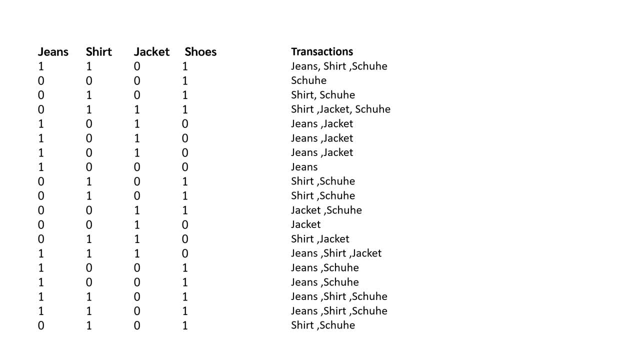 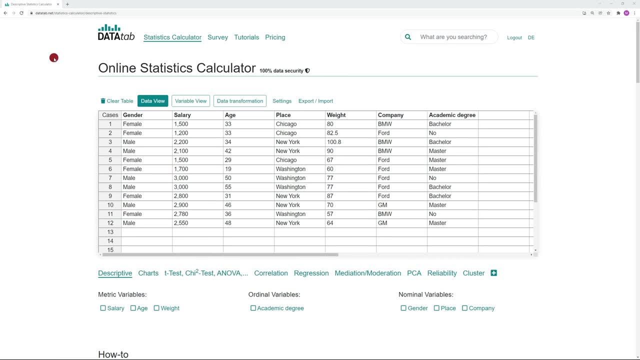 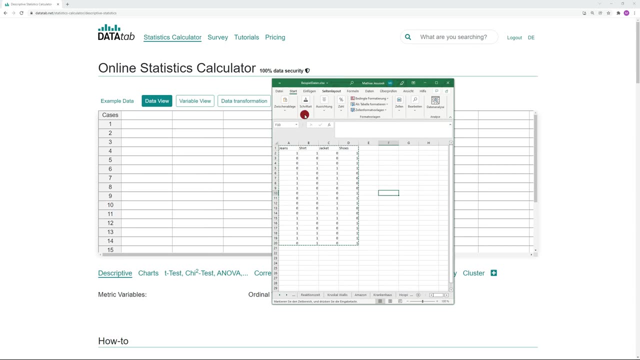 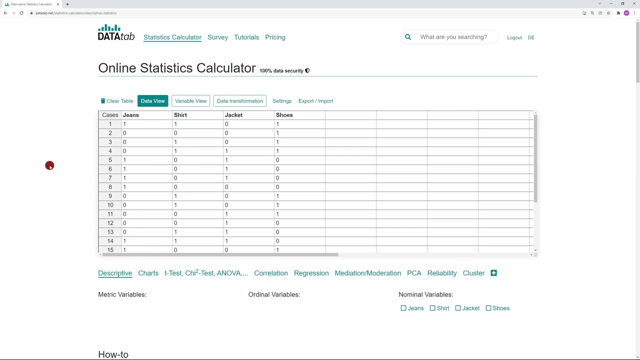 also interpret. let's first calculate a market basket analysis for this data. In order to do this, we go to datadepthnet, You find the link in the video description And you copy your data into this table. These are, of course, very few cases, but as an example it should be enough. 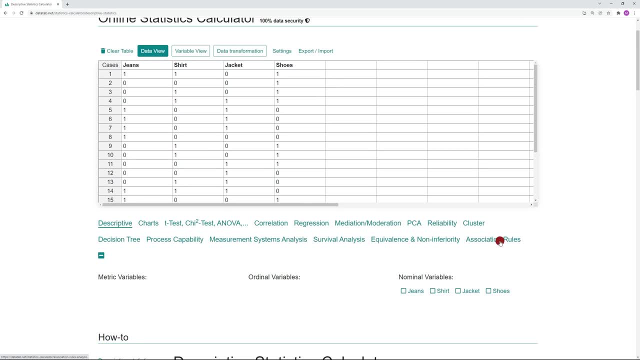 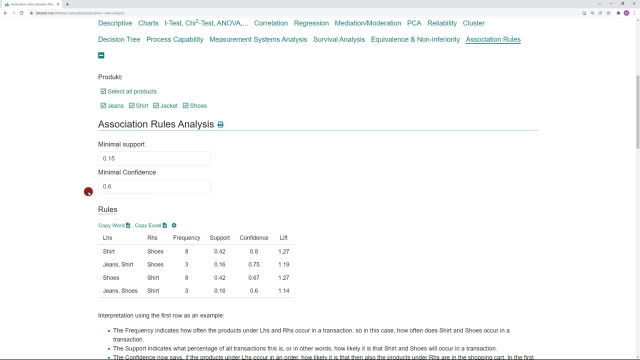 Then you click on plus and on the tab association analysis We go to the data depth And we copy the data into this table. And we copy the data into this table. We just click on all products. Now we can specify a minimum support and the minimum confidence. 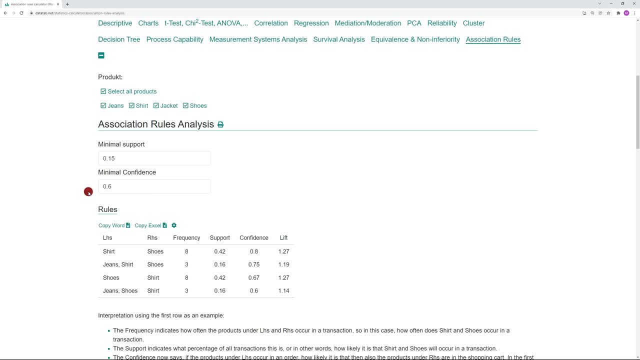 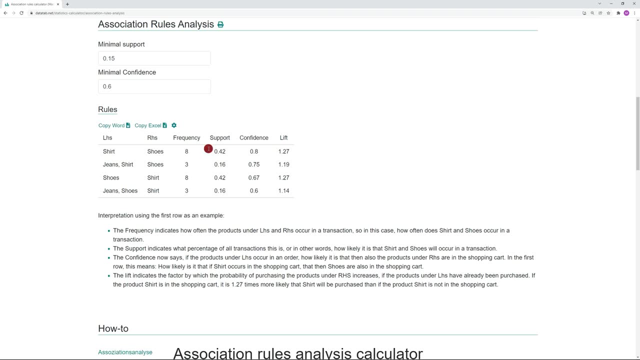 We will go through what support and confidence mean in a moment Here. below you get the results table And below the table you get an interpretation of the results from the first row. We'll go through this step by step. now, What is LHS, RHS, frequency, support, confidence and what is the lift? 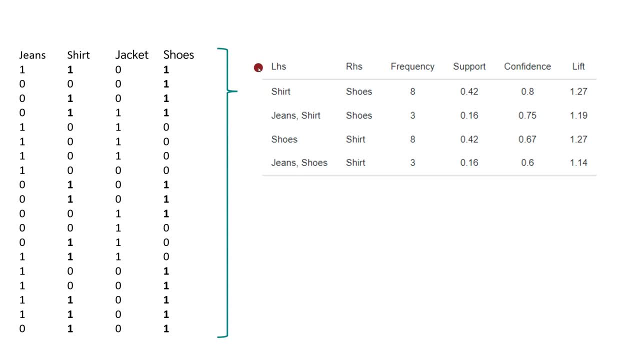 For this example, data Datadep has given us these association rules. Each row in this table is one association rule. The association rules are in the form: if the products under left-hand side are present in a transaction, then the products under right-hand side are also present, with some 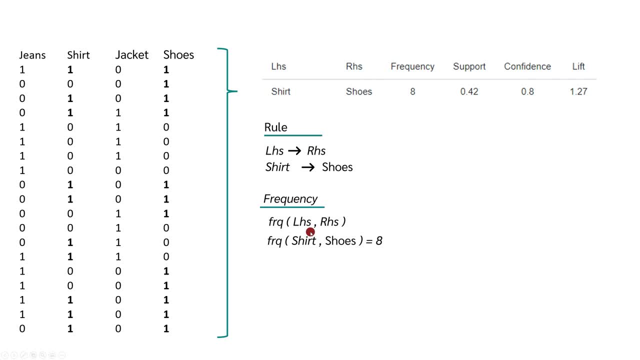 probability. Frequency tells us how often the products under left-hand side are present in a transaction. So in our case, how often does shirt and shoes occur in a transaction? So let's just count through in how many transactions both occur: 1,, 2,, 3,, 4,, 5,, 6,, 7, 8.. So the frequency is 8.. 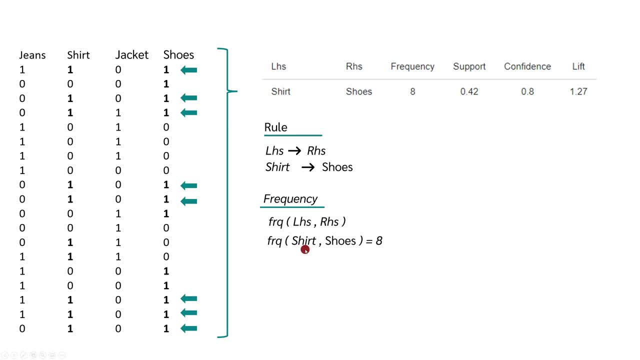 In 8 transactions shirt and shoes occur together. Support tells us what percentage of all transactions that is, or in other words, how likely it is that shirt and shoes occur in a transaction. So we just divide the frequency by the number of all transactions. We have 19 transactions in total. 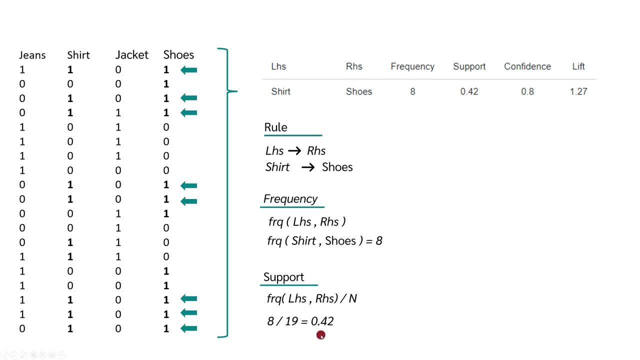 so we get 8 divided by 19,, which is equal to 0.42.. Therefore, the probability of shirt and shoes occurring in a transaction together is 42%. Confidence now tells us if the products under left-hand side occur in an order. 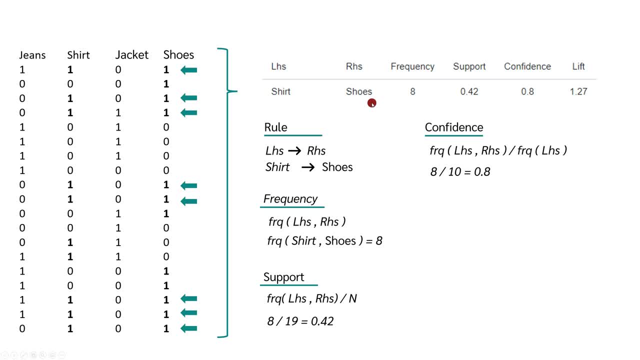 how likely it is that the products under right-hand side are then also in the shopping cart. In our example, this means how likely is it that if shirt occurs in the shopping cart, then shoes will also be in the shopping cart? We can calculate this by dividing the frequency. 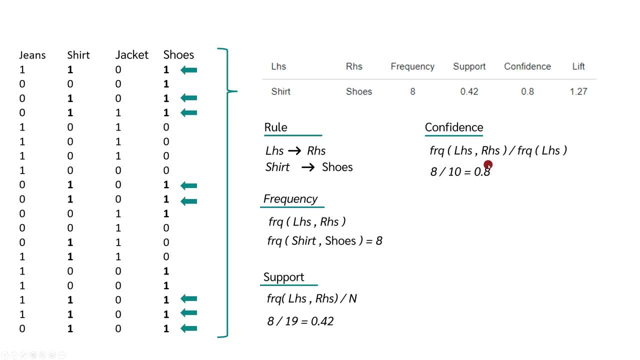 of shirt and shoes by the frequency of shirt. Similarly, the lift. The lift indicates the factor by which the probability of buying the products under right-hand side increases if the products under left-hand side have already been bought. So let's look at our example again. If the product shirt is in the shopping cart, it 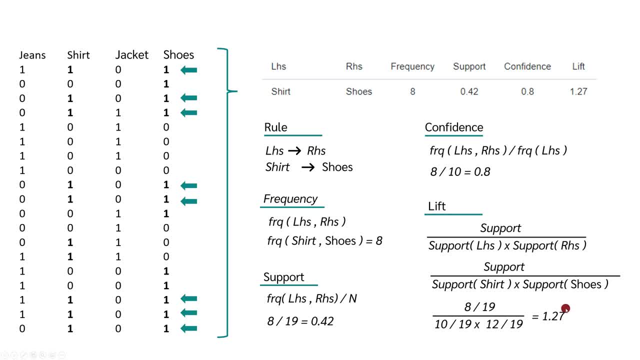 is 1.27 times more likely that shoes will be purchased than if the product shirt is not in the shopping cart. If you need support with the market basket analysis or you need an individual solution, just contact us. We can help you for sure.